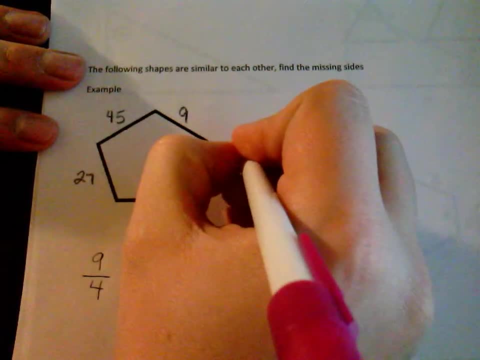 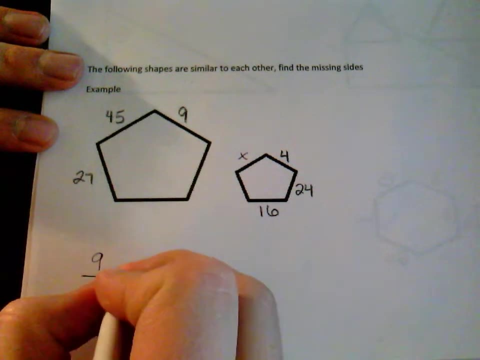 This 45 and this x, So I'm just going to label this one x. So 45 over x is like 9 over 4, meaning we do this 45 over x equals, or 9 over 4 equals 45 over x. 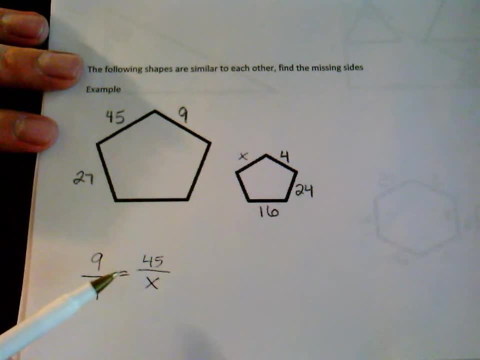 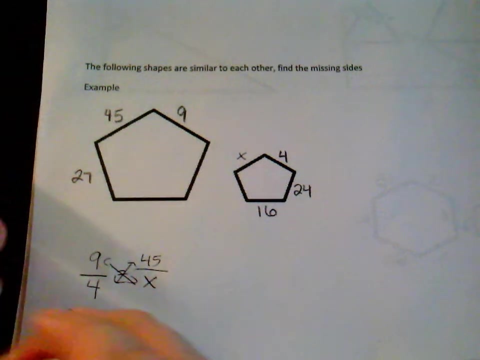 To figure this out first we need to cross Multiply. This becomes 9x equals 180.. To figure out what the side is now, we have to just divide by 9.. x gives us 20.. So we know if this side is 45,, this side has to be 20.. 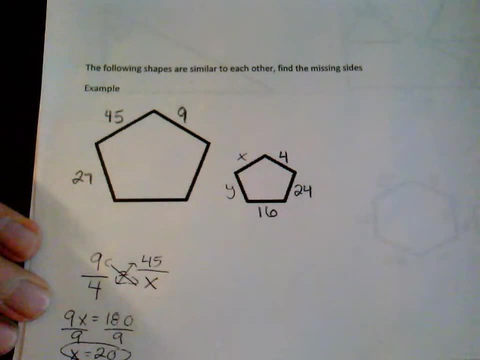 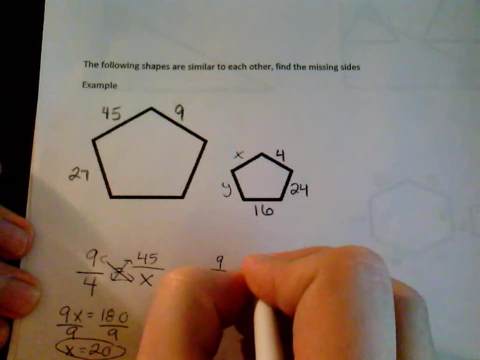 So we're going to multiply, So we're going to multiply. So now let's call this y and solve for that one. We know its comparable part is 27.. So we can say: 9 over 4 equals 27 over y. 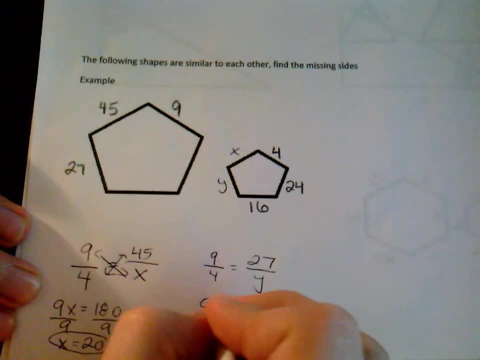 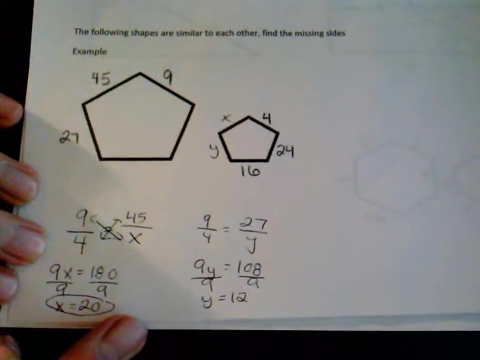 Cross. multiply again, So you get 9y equals 108.. If you divide by 9. y gives you 12.. So that means that this side right here is 12.. Now let's find z. Let's just label this one z. 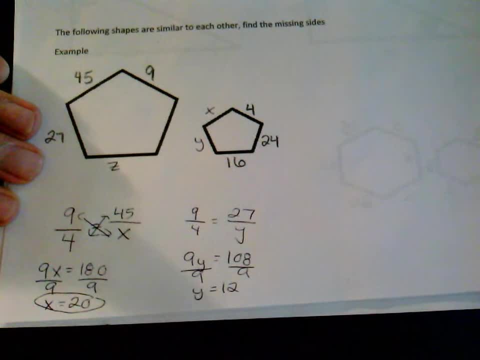 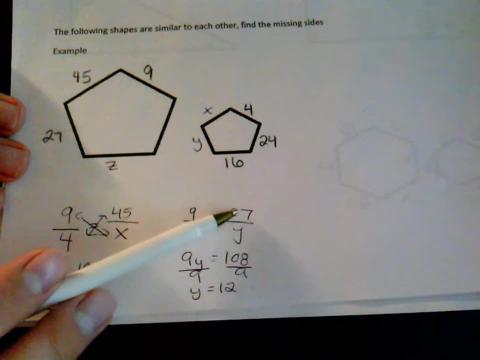 Let me put the little thing so you guys don't get confused. That's a 2. So z, So 16 and z. So instead of writing it as 16 over z, now it's going to be z over 16.. 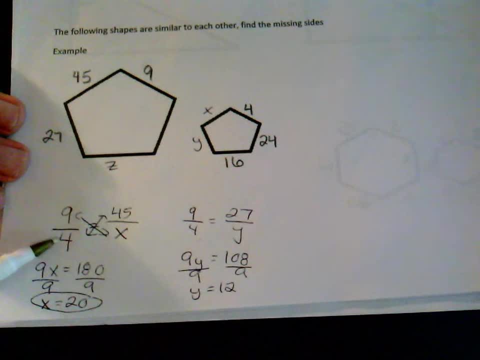 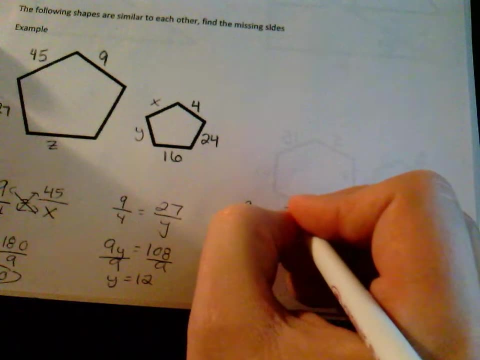 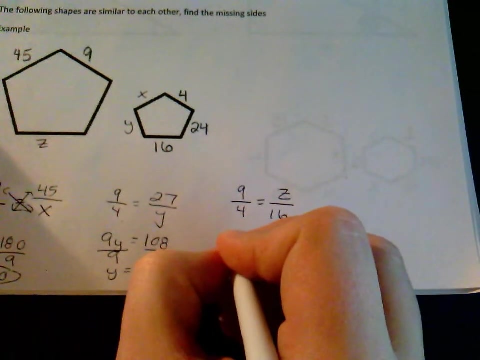 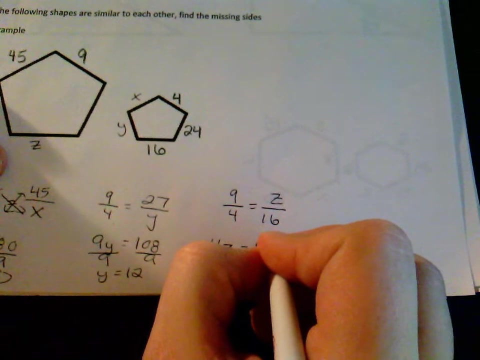 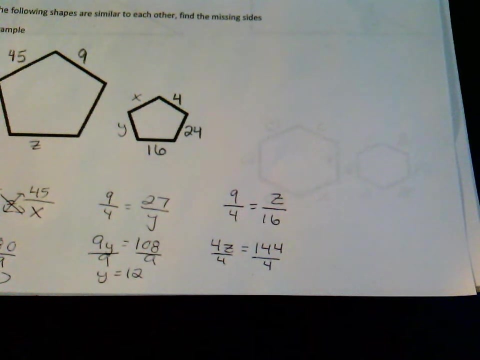 Because it's always the bigger over the smaller. So we've got to do: 9 over 4 equals z over 16.. So we cross, multiply, We get 4z equals 144.. If I divide by 4.. 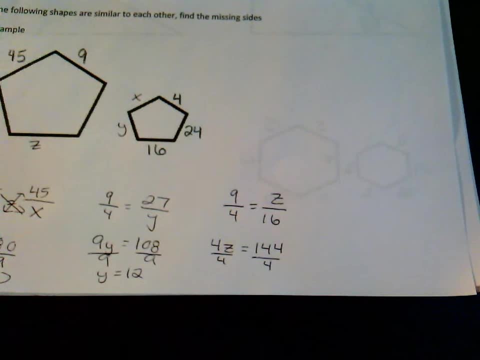 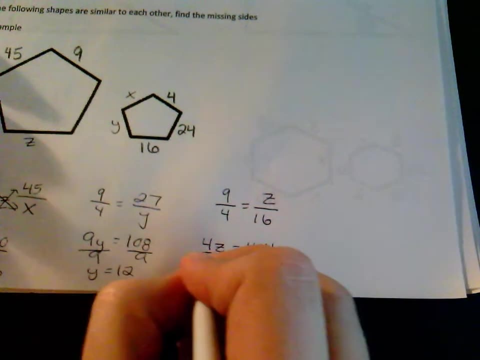 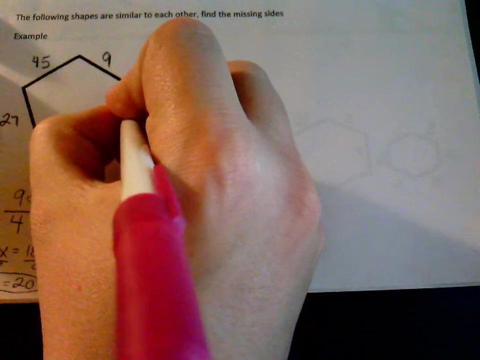 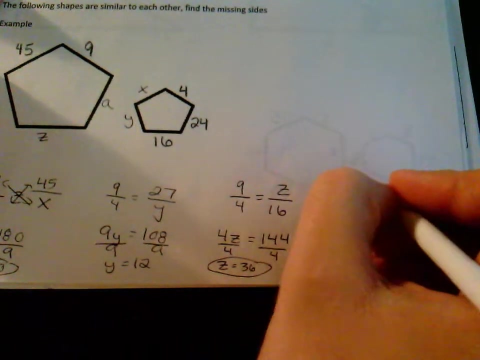 144 divided by 4 gives me 36,. so Z equals 36, and finally, I'm just going to label this last side A. okay, so let's figure out A. A is going to be 9 over 4, equals A over 24,.